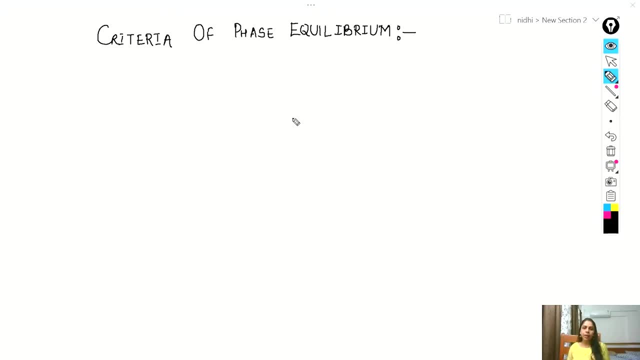 Now there are one more criteria, which is thermodynamic equilibrium. So for the thermodynamic equilibrium means because if there is a system and surrounding, there is the possibility of mass transfer. When the system interacts with the surrounding, there is a possibility of mass transfer. 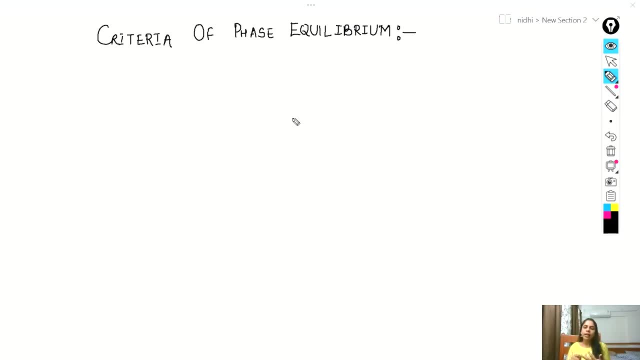 There is a possibility of heat transfer. There is a possibility of heat transfer, mass transfer and force transfer. So if your system should be in thermodynamic equilibrium, then temperature, pressure and another criteria, which is there is no mass transfer, should be fulfilled. 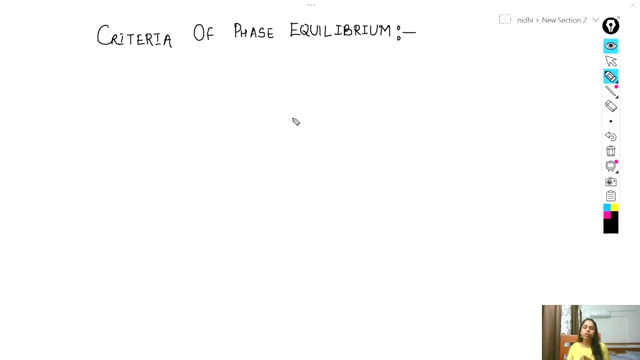 That means all three conditions should be fulfilled. So the thermodynamic equilibrium means there is no mass transfer, no mass interaction between the system surrounding, and temperature and pressure is also uniform throughout the system. So to establish the thermodynamic state or thermodynamic equilibrium state, the third criteria should be: it is very important and that is necessary to fulfill the third criteria. 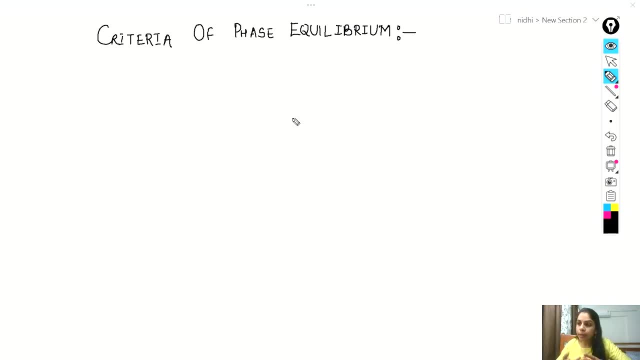 Now a system can interact with surrounding. In the case of irreversible process, a state of equilibrium is maintained throughout the process and the driving forces are only infinitesimal in magnitude. That means the driving forces for the reversible process is very small, The magnitude of the process is very small. 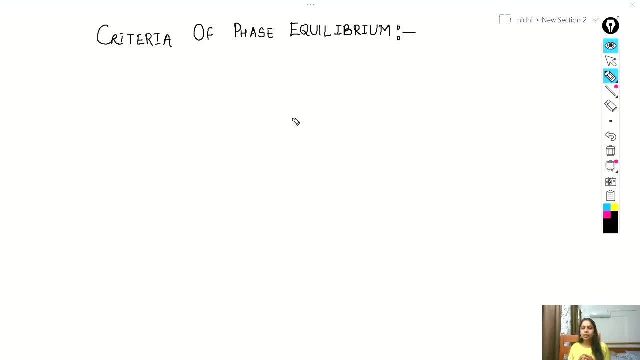 And due to these forces all the changes in the system will happen. They are also very small in magnitude, So the changes are also infinitesimal. In contrast, in irreversible process the driving forces are finite in magnitude and it cannot be reversed by infinitesimal changes in the external condition. 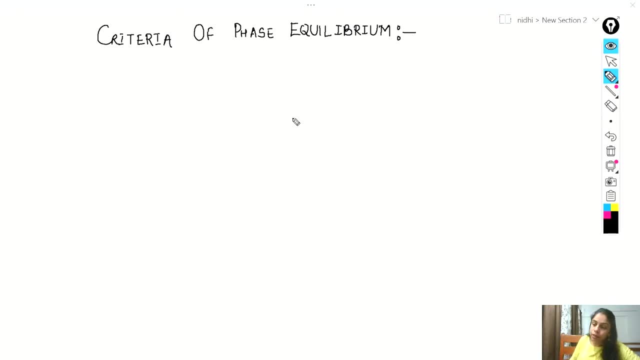 So, however, all irreversible process tends towards A state of equilibrium. So we have one equation, which is known as Clausius inequality equation. Inequality equation, and which this equation is: ds is greater than equal to dq by t. So, the first, we have the equality sign. 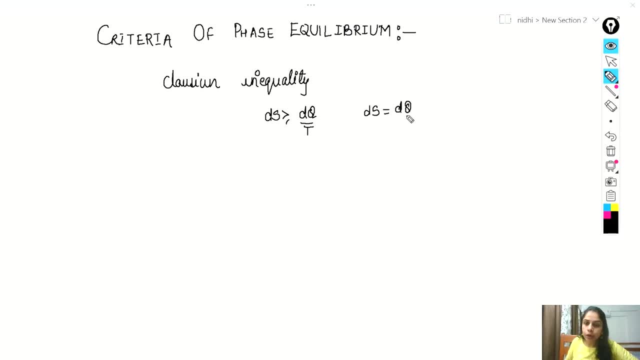 Equality sign refers to A reversible process which can be Reversible process, which can be treated as a succession of equilibrium state, and the inequality sign refers to the entropy change: change in entropy for a spontaneous process whose ultimate result would be an equilibrium state. Or you can say this: 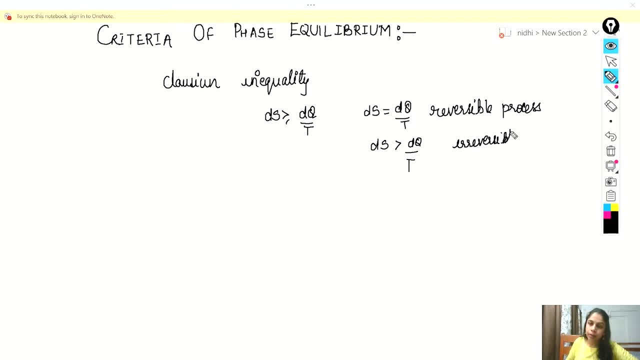 Irreversible process, Right. So now, from first law of thermodynamic, We know that Dq is equals to du plus Dw. So let's take this as the equation number one and this is the equation number two. So from equation number one, we can replace this dq by tds. you can write this tds. 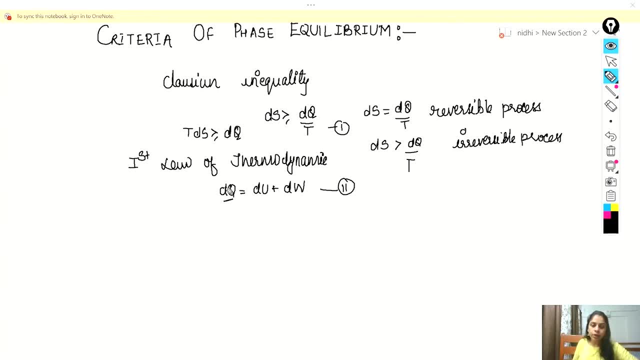 Greater than equal to Dq, So we can replace this dq by TDS. So just replace it so TDS is greater than equal to du plus Dw, Or rearrange this du is u less than equal to TDS minus DW, and this DW you can replace by PDV, So DU is less than equal to. 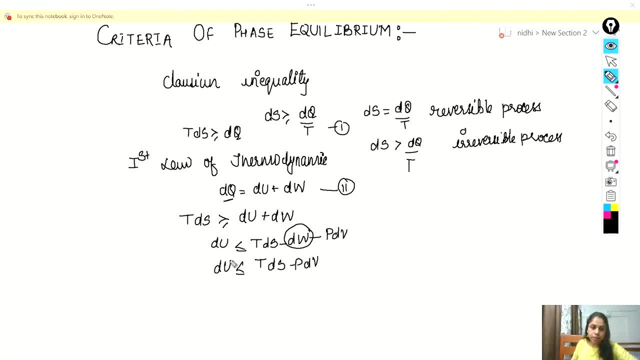 TDS minus PDV. So this, you can see, this is. this equation is the combination of first and second law of thermodynamic applied to a. this is the third equation. So you can see, this is the. this equation is the combination of first and second law of thermodynamic applied to a closed system. 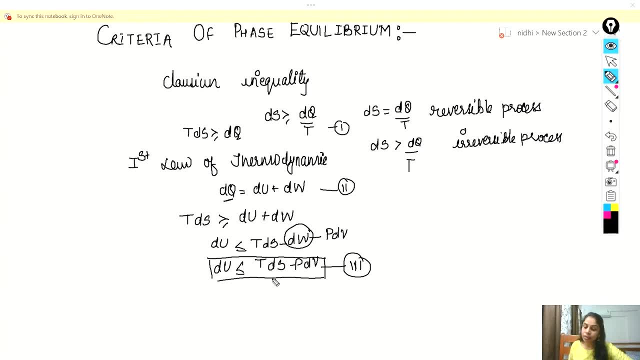 which interacts with its surrounding through a heat transfer and work of volume displacement. Now, here you can see. this equation is valid for cases where external pressure- you can see here the external pressure- is the only force, pressure is the only force, or Kaisa work, milgram ko. 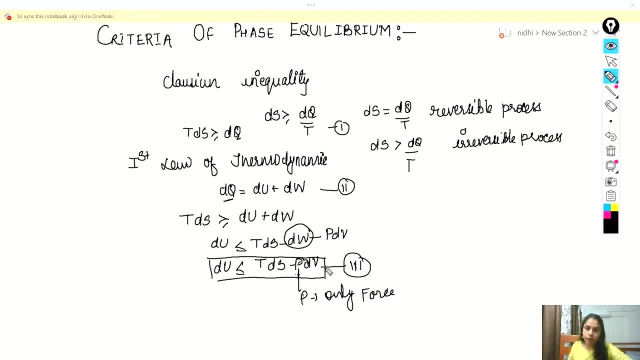 Expanded Expansion work. milgram only force and work Kaisa milgram, because kya ho raha hai? volume change ho raha hai. Ja, volume change ho raha hai to kaisa work milta hai. We are getting the expansion work. 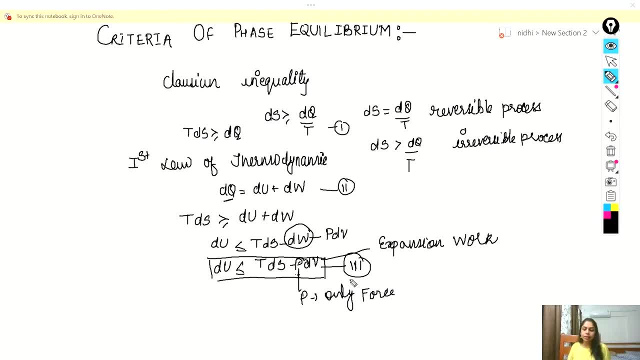 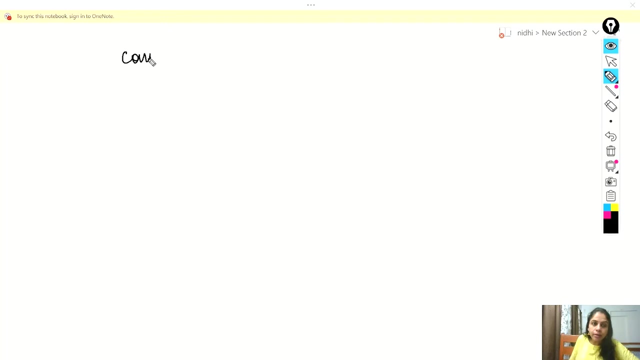 Okay, so this is the general equation which we get from the, which we consider as a general, for general equation for the phase equilibrium. Now here we have three cases. now let's let's discuss. the first case is at constant, at constant internal energy and volume. right, so here we can see the internal energy and volume of constant as we need to be. 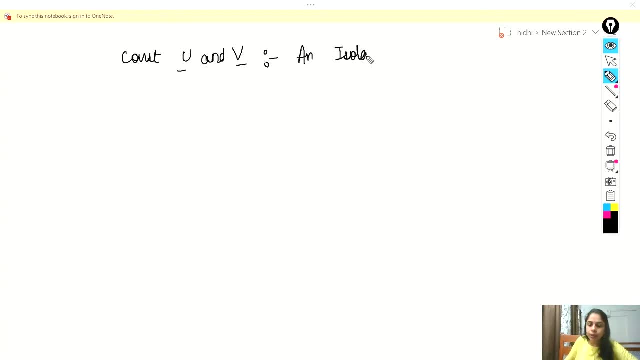 consider an isolated system. isolated system because isolated, this system does not exchange mass heat or work with the surrounding. so this equation we have. equation d. third equation, du, sorry, dq. first, from the first law of thermodynamic we have: dq is equals to du plus dw. so if internal energy and volume is constant, that means your system is isolated. 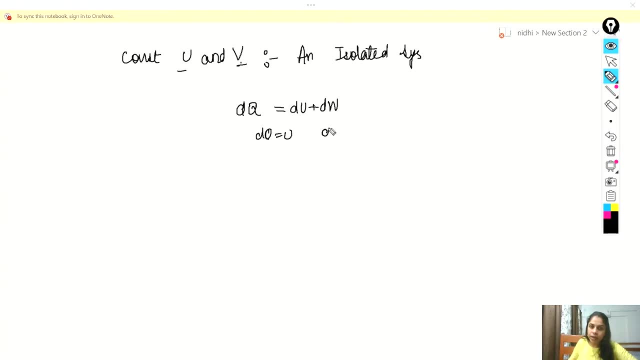 system, then dq is equal to zero and there is no, no work. so dw is also equal to zero. so once dq and dw is equals to zero, hence du also equal to zero. a well insulated vessel of constant volume would closely approximate this behavior, this equation number. we have equation. 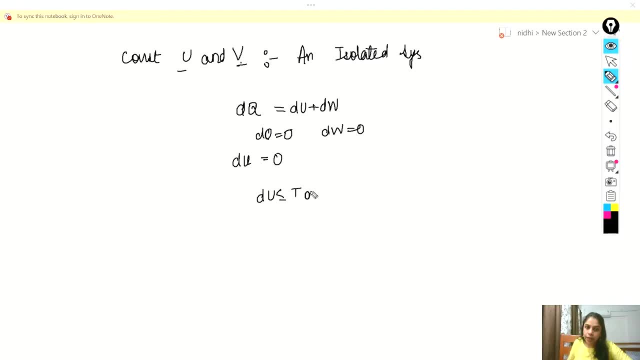 number three: du less than equal to tds minus pdv. right, this is our equation number third. so here are in this case, in this case du is equals to zero and dv is also equals to zero because we have closed system, so volume will also not going to be changed. so if du and dv is equals to zero, 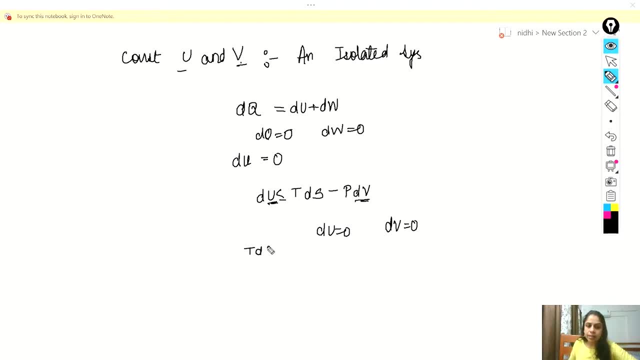 then we have: tds is greater than equal to zero and ds at constant internal energy and volume, is greater than equal to zero. so in this equation- this is the first 항 and this is other Subtitle- is constant in a reversible process and increase in a spontaneous process occurring in a system. 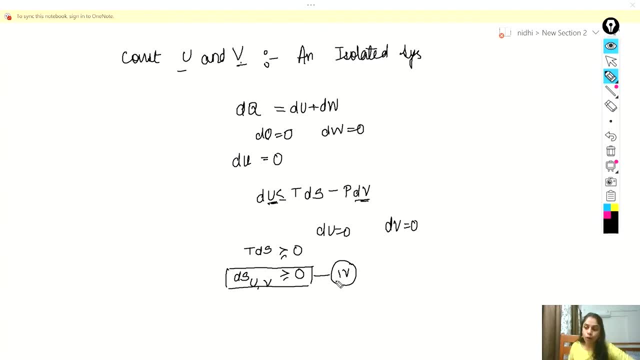 at constant internal energy and volume. right. so here again we have two signs: HR inequality sign and equality signs. rope 같아요 to signиг you sign. and Equality sign refers to the reversible process, and this sign equals to second sign in our reverse process. so this is both. so this equation did not change the expression here. 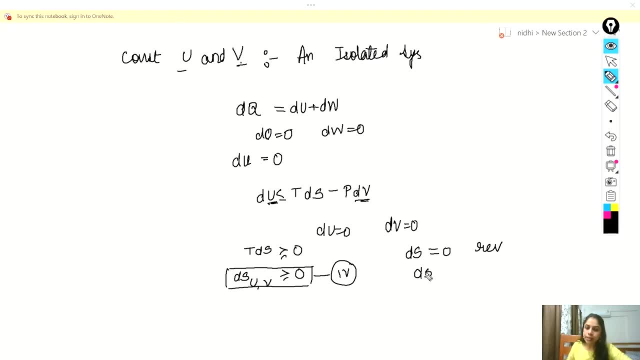 process. An inequality sign refers for the spontaneous process. So, since an irreversible process leads the system to an equilibrium state, the entropy is maximum. at equilibrium No further spontaneous processes are possible. So at equilibrium, entropy is maximum and when no further spontaneous processes are possible. Now let us discuss the second case. 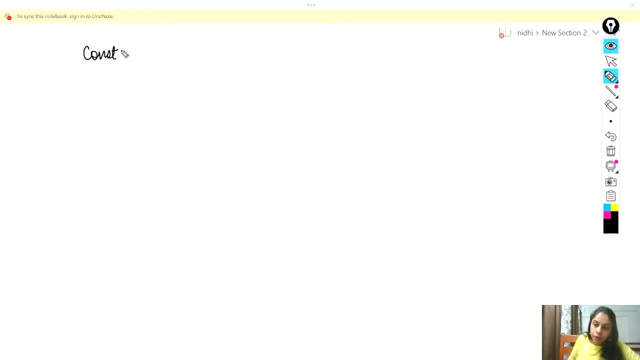 at constant temperature and volume. So we know that helmets from helmets, free equilibrium, no further spontaneous processes are possible. So at equilibrium, entropy is maximum at equilibrium. So at equilibrium, entropy is maximum at equilibrium. We know that A is equals to U minus TS. So just rearrange this. So U is equals to A plus TS Differentiate. 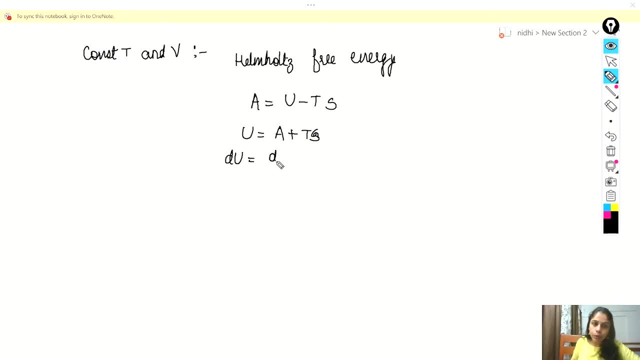 this equation, So we will get: DU is equals to DA plus TDS plus SDT. And from equation number third, we know that that DU is greater than TDS plus SDT, So we know that that DU, than sorry, less than equal to TDS minus PDB. so we can substitute here over here. 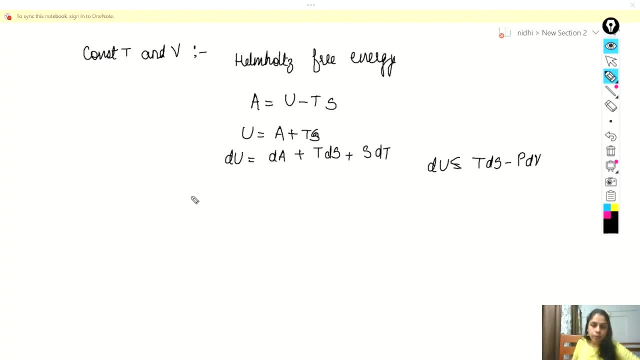 this. so in place of DU you can substitute TDS minus PDB, right greater than equal to DA plus TDS, plus STT. so TDS, TDS cancel will get cancelled and then we have: DA is less than equal to minus PDB, minus SDT. and condition k- mrs case key- at constant, at constant. 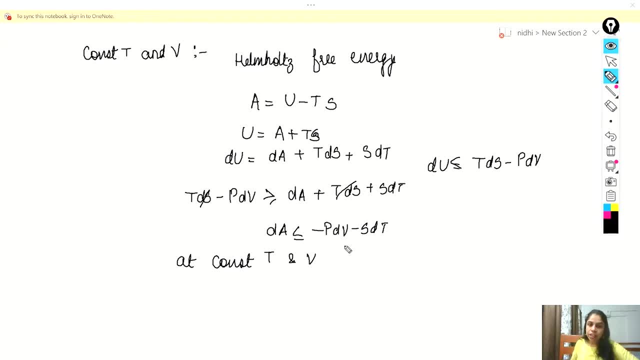 temperature and volume. so change in volume and change in temperature will be equal to zero, right? so da change in Helmholtz for every energy at constant temperature and volume less than equal to zero. and this is the second criteria of of for phase equilibrium. so here in this equation, let's 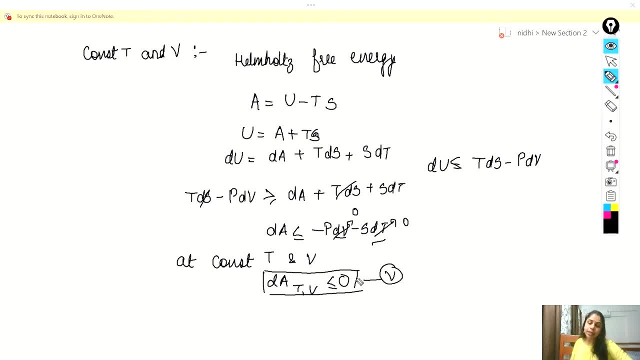 take this as the equation number five. so equation five means that the spontaneous process occurring at constant temperature and volume is accompanied by decrease in the work function. right, Helmholtz, free energy. I make a without a. it tell us about the work function you approach work. 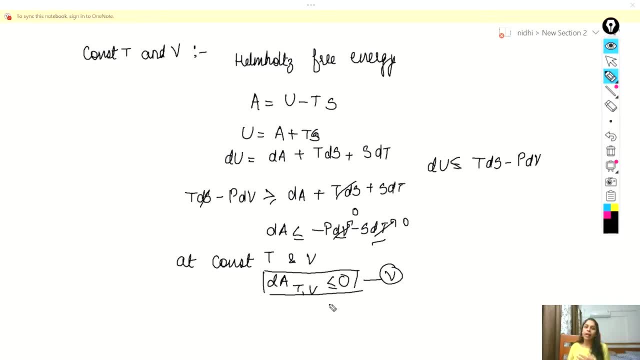 here how much work you have to do and how much work you have to do and how much work you have to do. you are getting from the useful work we are getting from the system right. so the spontaneous process over less inequality sign over. we know that equality sign refers for the reversible process. 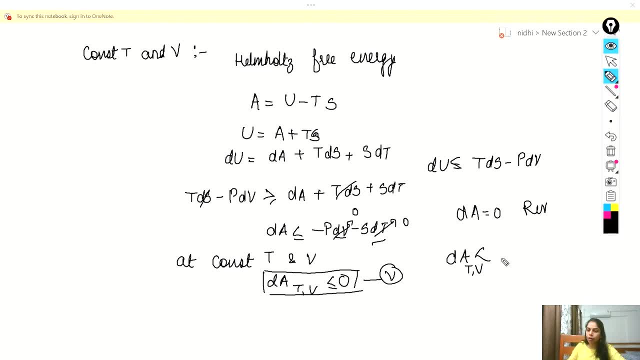 right. inequality sign at constant temperature, volume refers for the spontaneity, spontaneous process, so spontaneous cover of the system when work function. yoga vote negative over right. so a this equation, this relation means the spontaneous process occurring at constant temperature and volume and accompanied by a decrease in the work function and consequently in a state of 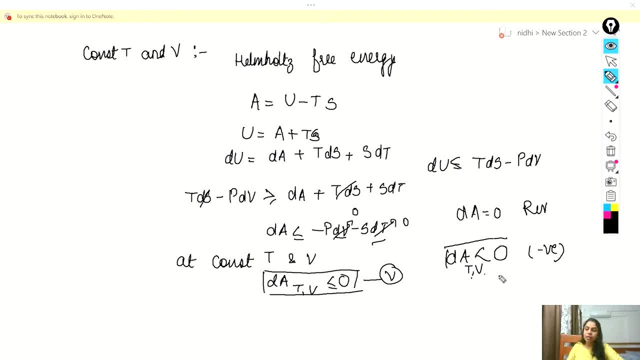 thermodynamic equilibrium. under these conditions the Helmholtz free energy or the work function is. Helmholtz free energy or work function is minimum at these condition, at constant temperature and volume. so this is the second criteria for the phase equilibrium. now let's discuss the last. 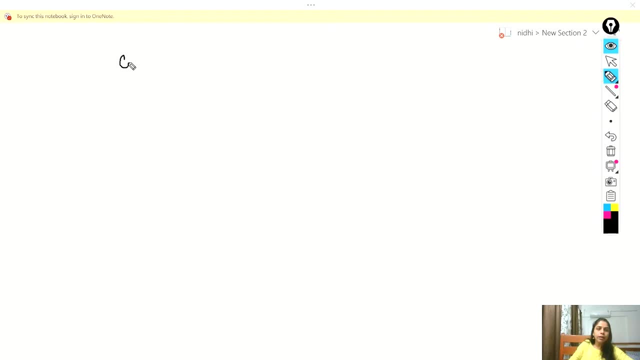 criteria for the phase equilibrium, which is at constant temperature and pressure. so we know that that the Gibbs free energy is the function of temperature and pressure. so we have have gives free energy. so g is equals to h minus ts. and enthalpy we know that h is equals to u plus. 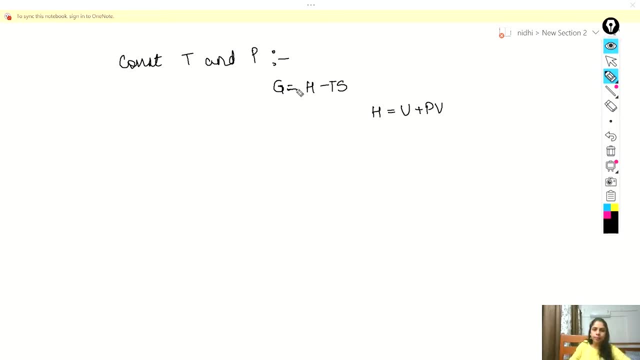 pv, so you can just substitute here. so g is equals to u plus pv, minus ts. now just differentiate this equation above equation. so dg is equals to du plus pdv, plus vdp, minus tds, minus sdt. right, so from equation number. third, we know that that du is less than equal to tds minus pdv, so just rearrange this so du is. 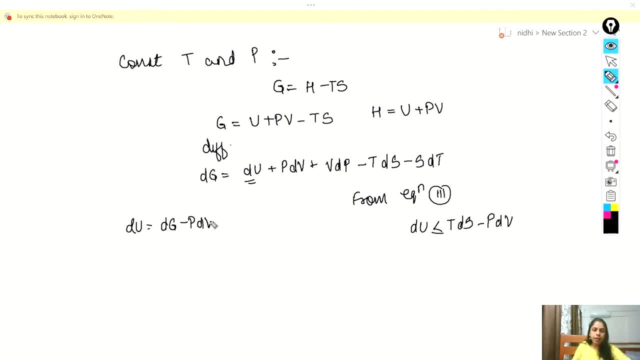 equals to dg minus pdv, minus vdp plus tds plus sdt. so in place of du we can substitute tds minus pdv, dg minus pdv minus vdp plus tds plus sdt. so mine pdv pdv cancel over, cancel over, and then we have dg is less than equal to sdt, right, so we have vdp minus plus. 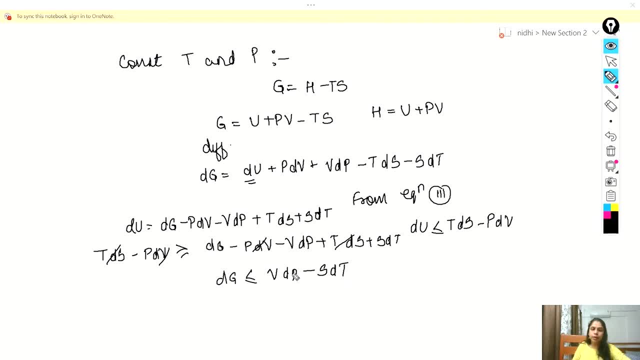 sdt. so our condition is at constant temperature and pressure. so change in temperature and pressure can. temperature and pressure is constant for this case, so change in pressure and change in temperature will be equal to zero. so dg at constant temperature and pressure less than equal to zero. 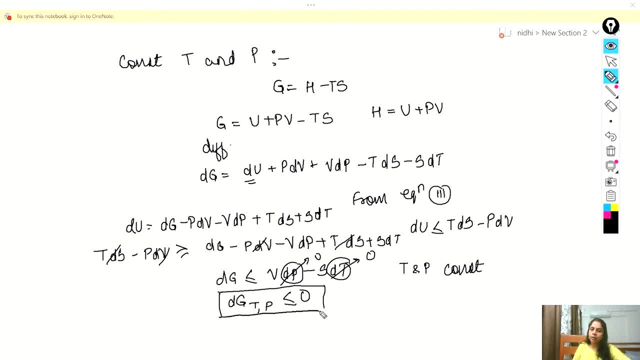 and this is the very important phase- equilibrium criteria and this equation let's take. this is the equation number sixth equation. this equation means that the free energy either decrease or remains unaltered, depending upon whether the process is spontaneous or reversible. right, if your process is reversible, then dg is unaltered. 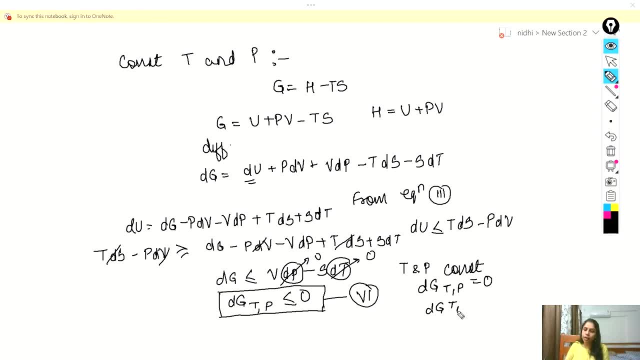 it is equal to zero and if it is spontaneous then it will be equal less than zero. that means spontaneous. if your process is spontaneous, then the change in Gibbs free energy will be equal to zero, will be negative, and if it is positive then your process will be non-spontaneous. if dg is 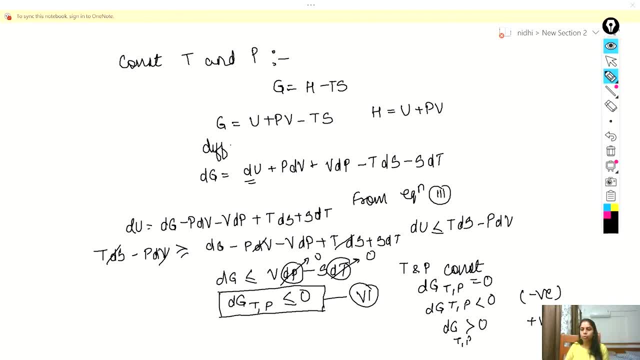 greater than zero, then your process is non-spontaneous process, since most chemical reaction and many physical changes are carried out under conditions of temperature, constant temperature and pressure. so this equation is commonly used criteria of thermodynamic equilibrium. it also provides a very convenient and simple test for the feasibility of a process, and no process is possible which results in an 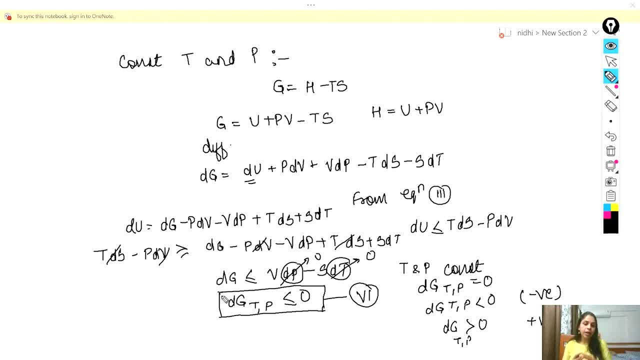 increase in the Gibbs free energy of the system. other Gibbs free energy increase or a positive, then will process possibly need physically me. so for the feasibility Gibbs free energy will be process, keep feasible. honey Kelly, a process Gibbs free energy can see on a chair, negative on a chair, decrease on a chair. so 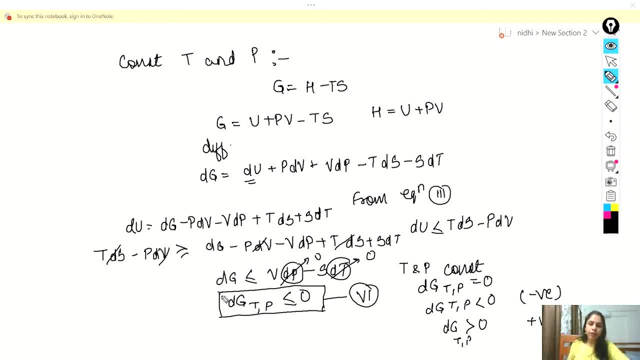 it will be any process. it just curious who cha Krishna ака P hi and volume and said a change in propriety and 4? these are the kids we are going to discuss the three phases�isine entropy always increases. Second criteria is the Helmholtz free energy is less than.